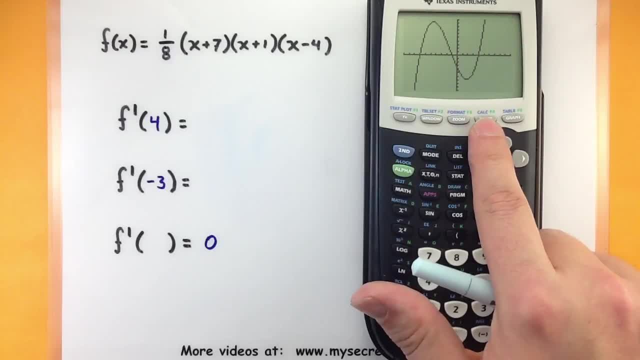 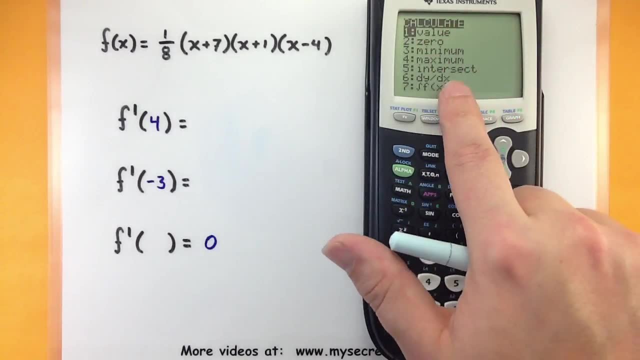 value. Above your trace button it says calc, in usually a different color. so press your second button and then that trace button and you get lots of different options. You want the sixth one that says dy, dx. that is for your derivative. So scroll down and select. 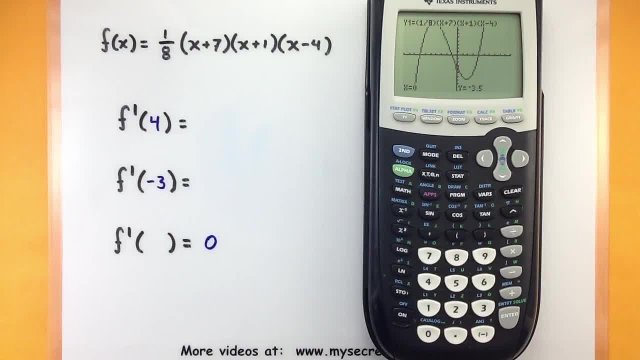 it and press enter. Okay, Now, after this point the calculator wants you to give it some sort of value wherever you're looking for that derivative. So I'm going to type in the number 4 here, so that little x equals 4 shows up, then I'll press enter So it looks like it's giving me the 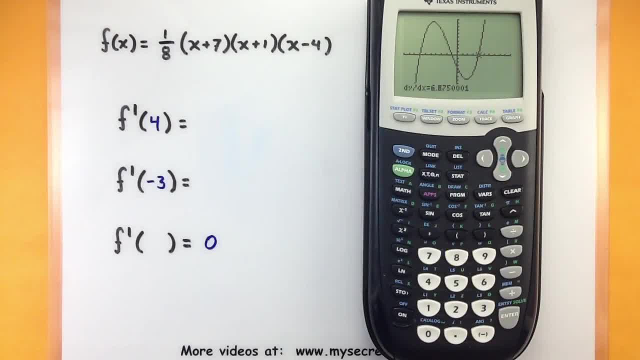 value of 6.8750001.. Sometimes it goes through a numerical method where it's just estimating that limit, so I'm going to chop this off and say 6.875.. All right, let's do another one of these. Let's find the derivative at negative 3.. So 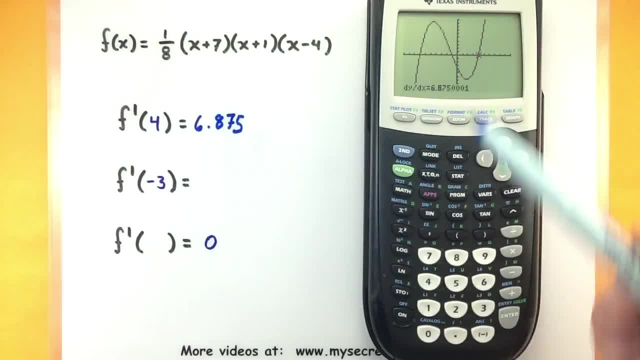 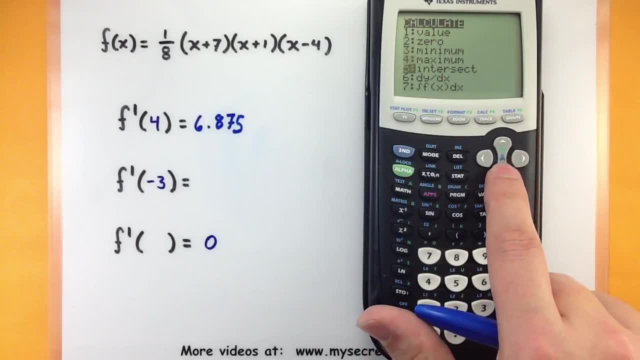 this is on this part of the function. you can see that it's decreasing, so we should get a negative number. So second calc: go all the way down to dy dx, press enter and let's give it that value of negative 3.. So type in negative 3,. so x equals negative 3,. 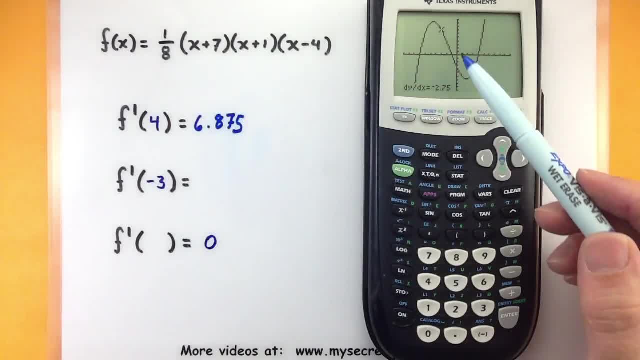 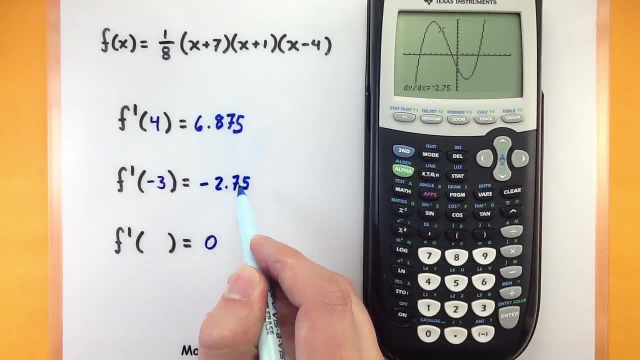 yep, that's good. Press enter, Okay, And it looks like this is giving me the value of negative 2.75.. There we go, Awesome. Now, every once in a while, you might want to work backwards. In other words, what value would the derivative equal 0?. 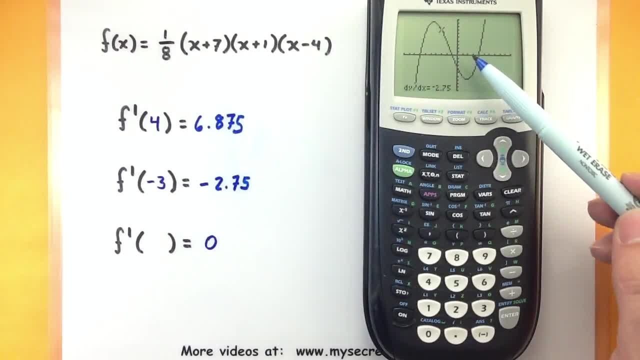 Well, for our particular function it looks like it would happen in two different spots, Say either at this local maximum or at that local minimum. Now, unfortunately you can't just type into your calculator here. hey, find where the derivative is equal to 0,. 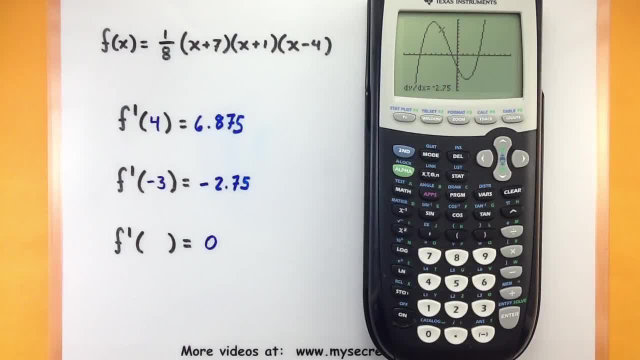 but you can use this feature to kind of estimate where that is. So let's take this first one. So I notice that this minimum- it looks like the derivative- is equal to 0, maybe somewhere around 2.. And I can check if that is the case by actually just checking its derivative there. 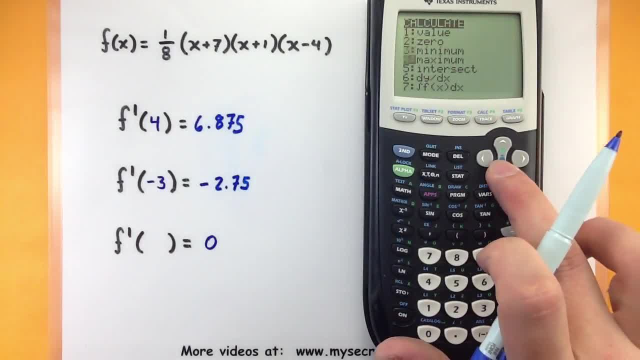 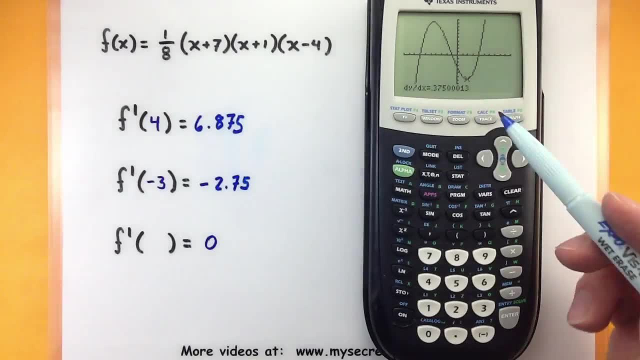 So I'm going to 2nd calc, selecting the derivative, and let's see what the derivative is at 2.. So x equals 2.. You know what? It's pretty close. It's close to 0,, but not quite. 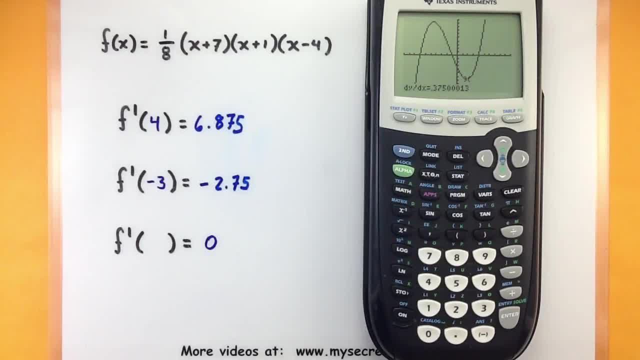 But if I was just, you know, trying to ballpark and say: eh, it kind of looks like the derivative is 0 at 2, you know, this might be a good estimate. All right, If you want to find the exact value of where it equals 2,. 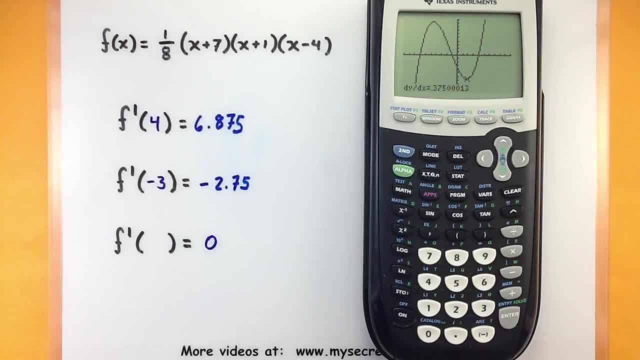 then you want to use, say, the maximum or the minimum function. So let's say I'm going to go to 2nd calc and that little bottom part it looks like it's a minimum, So I'm going to select number 3 for minimum. 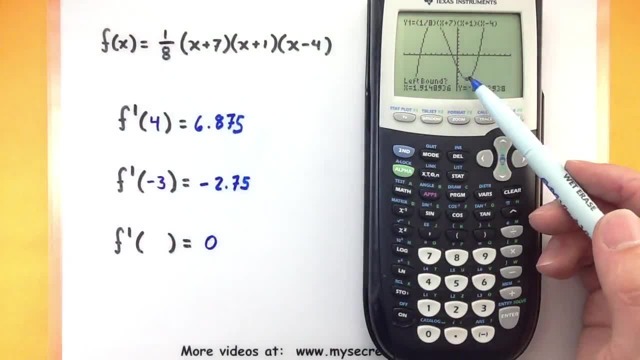 And now I have to give it a few other values. So this minimum point: it looks like it's somewhere around 2.. I need some point on the left side and on the right side of 2.. So let's select 1 for our left bound. 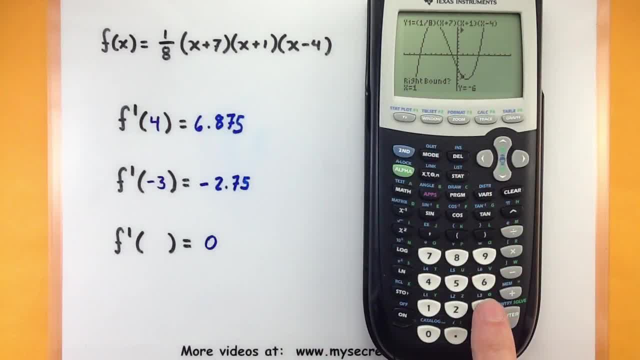 So x equals 1 for the left And let's select 3 for the right bound, And our guess is somewhere in between. Let's go ahead and put that 2 in for our guess. So the computer will work for a bit. 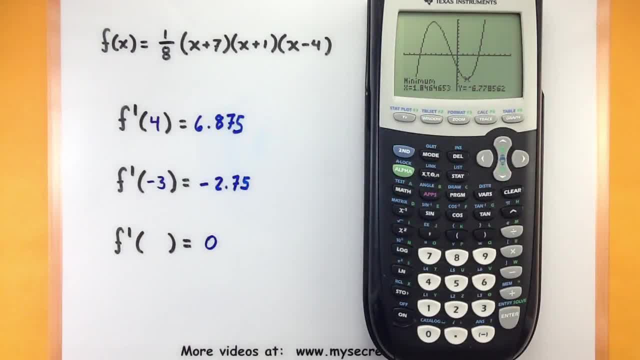 And then it comes up that the minimum is somewhere around 1.8.. Maybe about 1.85.. So we'll put that in as the place where our derivative is about equal to 0.. OK, So if you just want to directly compute what the derivative is at a point. 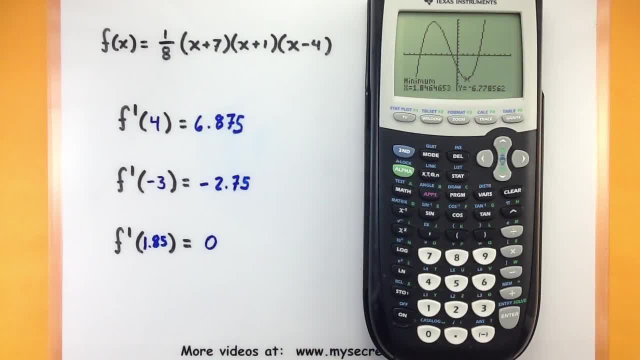 you've got a nice function for that and it'll give you a good estimate. If you want to work backwards, then oftentimes you have to think of some other tools that will actually give that to you. OK, So hopefully that helps out. If you want to see some more math videos, please visit MySecretMathTutorcom. 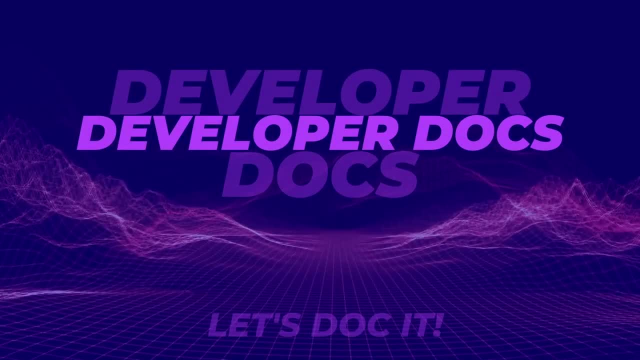 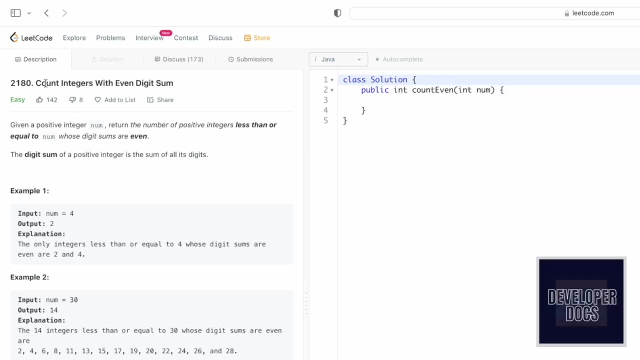 hey guys, welcome to a new video. in today's video we're going to look at a leetcode problem and the problem's name is count integers with even digit sum. so in this question we're given an integer and we have to return the number of positive integers less than or equal to num. 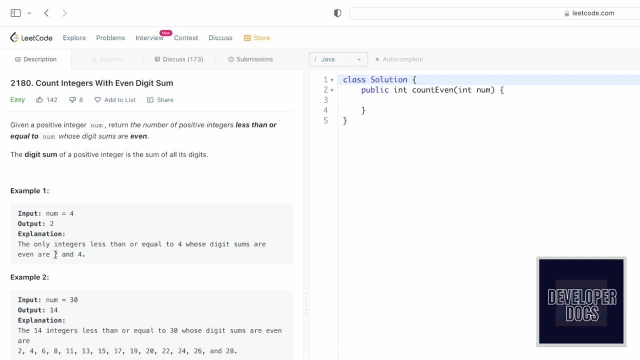 and 4, which are within the range, because some of all the digits in 2 is equal to an even number and sum of all the digits in 4 is also equal to an even number. in this example, the limit is 30 and there are 14 integers less than or equal to 30, whose digit sums.